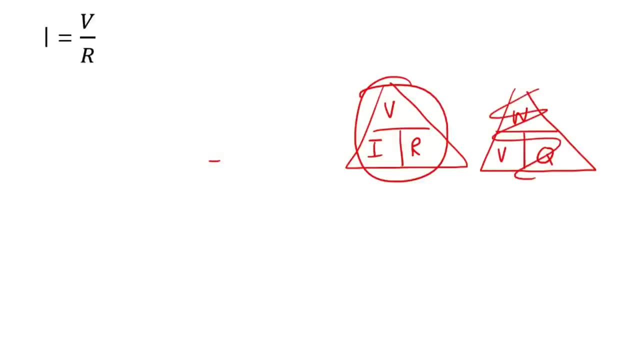 these ones for now. Okay, let's actually just get rid of them completely. Of course, we need to still know them, But when we are looking at electrical circuits, this is the most important one now in grade 10,, grade 11, and grade 12.. So let's just recap how these formulas 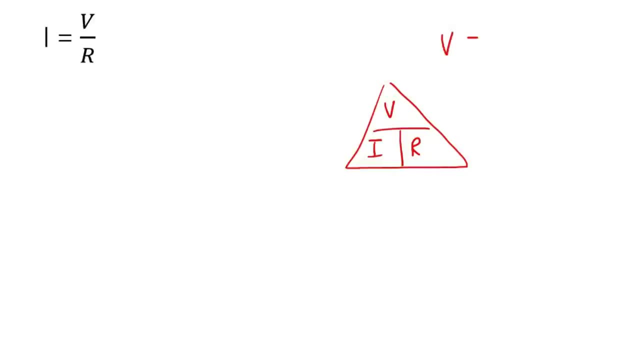 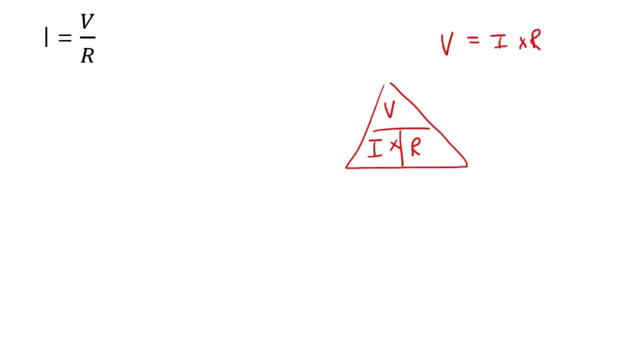 that are at the bottom. Okay, so that's a formula we need to know. If we are looking for I, then you got V at the top, R at the bottom, V at the top, R at the bottom, And then, if you are looking for R, 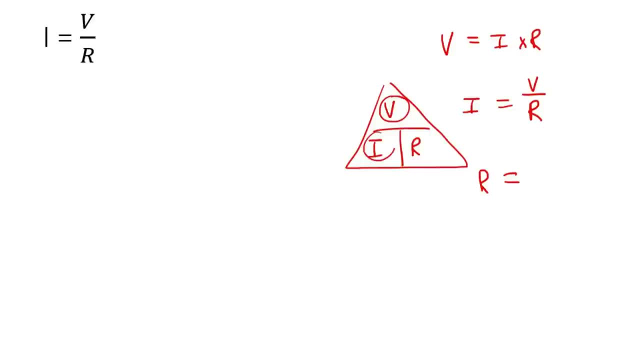 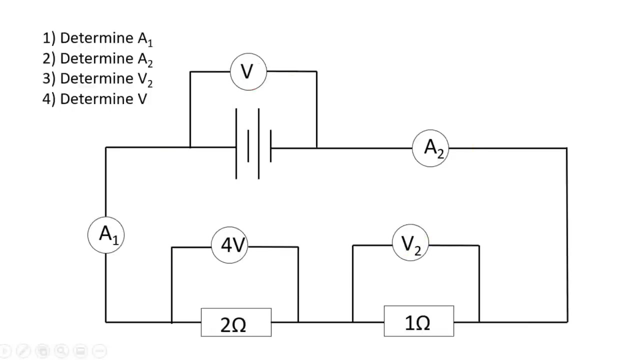 then you would say: V at the top, I at the bottom. Okay, so these are the three formulas that we will be using in this lesson. Now, this lesson is going to start off pretty basic, where we've got things like this, But then it's quickly going to start getting more complicated. 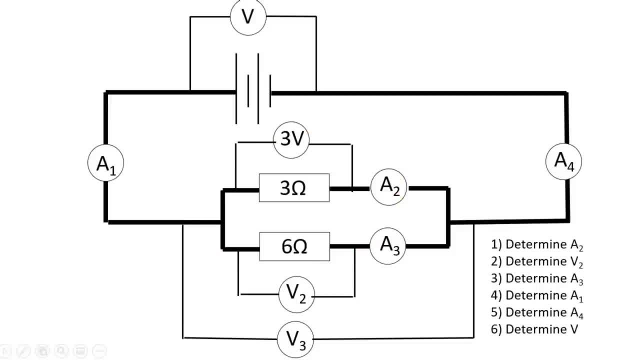 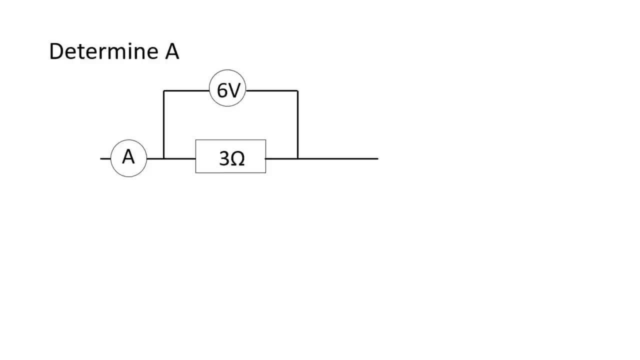 where we have series circuits and then we're going to have parallel circuits. So stay tuned for all of it It's going to get more difficult as we go along. So here's our first question Now. this one says: determine A. Now, A is a ammeter which is current. So if we look at those formulas, 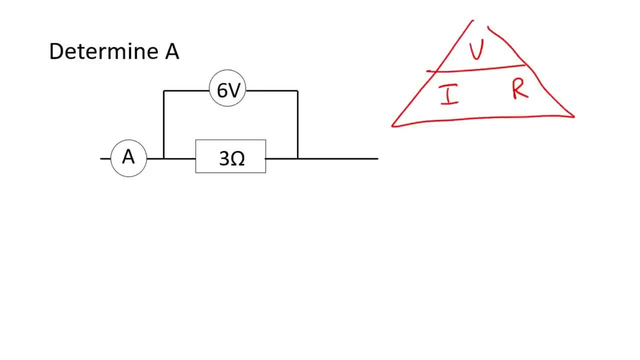 with the V, we're going to have a series of circuits. So we're going to have a series of circuits. So we need to know that when they're asking you to calculate A, then you need to remember that A is current. So that's the I. So we could then say that I is equal to V over R, because that's what 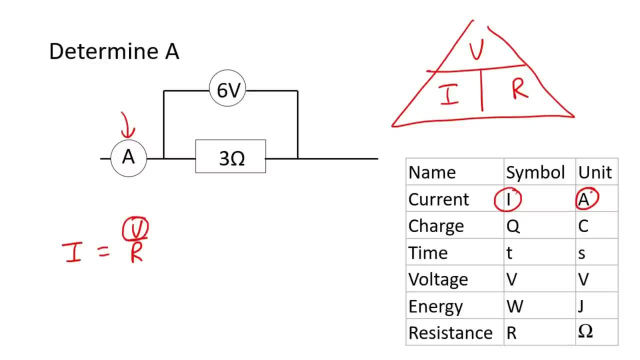 you get if you use this formula. So we need a voltage value. Okay, so we've got a voltage value of six. Now it's not going to be this easy, but I'm just building you up from the basics Now. 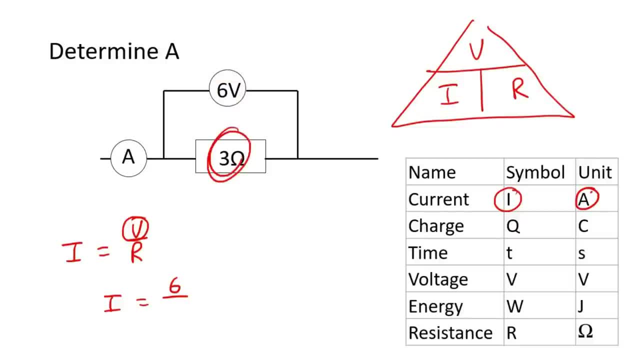 this voltmeter is connected, So this V and this R, they can go together. So you've got to look out for that, And so that's going to give us six divided by three, which is two amps, And so this would be two amps, Okay. 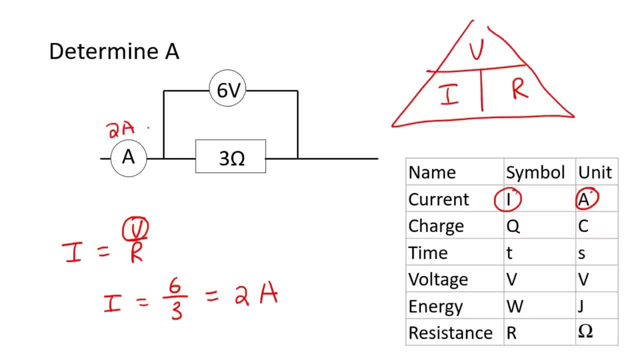 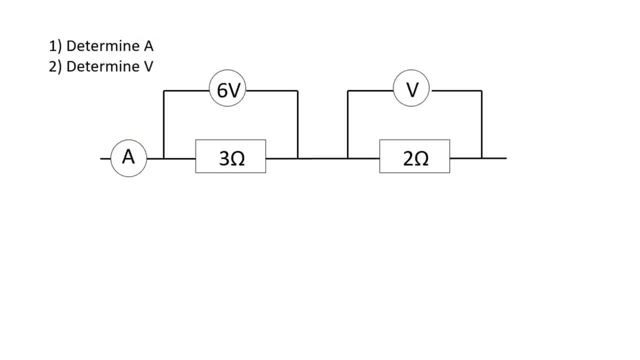 so that's quite easy. I understand that, But we're going to make it more complicated as we go along. Here's the next one. So the first question says: determine A. Now, A is a current, So we know that thisalleünh is constant, And so it means that this is an. 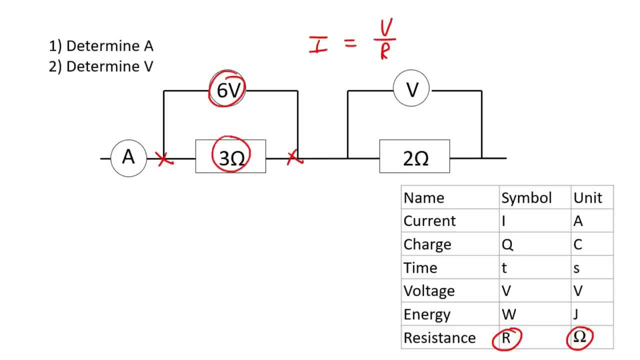 hour resistor and the current current yineither. Of course, we won't just choose any V and any R. For example, you can't just choose this V and this R. no, they need to go together. So this V is connected. across this resistor. Okay, And I didn't mention this in the previous slide, but remember that resistance is the symbol over here. Okay, and I didn't mention desimbly: This is a resistor, so these two are allowed to go together. So if we use I equals to V over R, we could say that I is equal to V over R for this resistor. 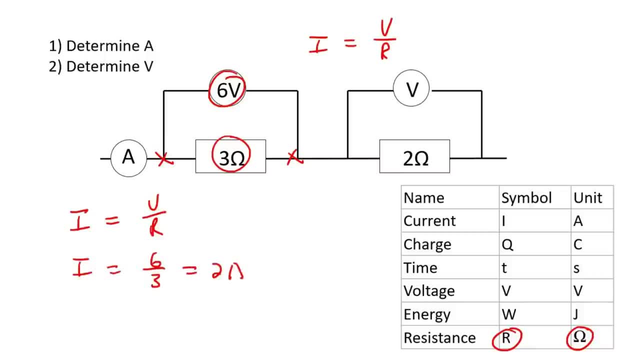 visa. we can conflict that with each other. So this is a DMR V, that is a vector resistor. ToZZить that in the графic pass, hallwayelson it is Landscape relationship to the nuclear recycle is equal to six over three and that would give us two amps okay. so that means we have two amps over. 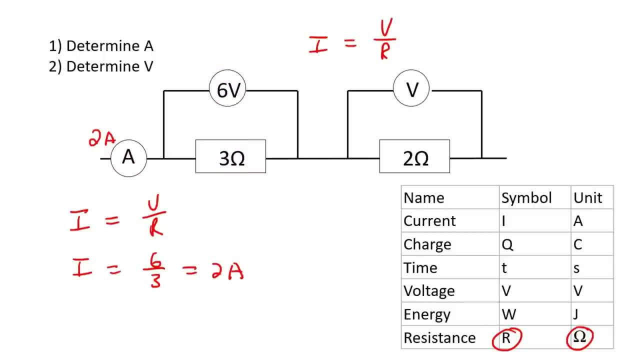 here now. the next question is: determine v. okay, so this is a volt meter over here. so if we use our triangle again, so v i r, then to calculate v, you multiply i and r together. so what that means is we need some type of current, okay, and we need some type of resistor so we can see which resistor. 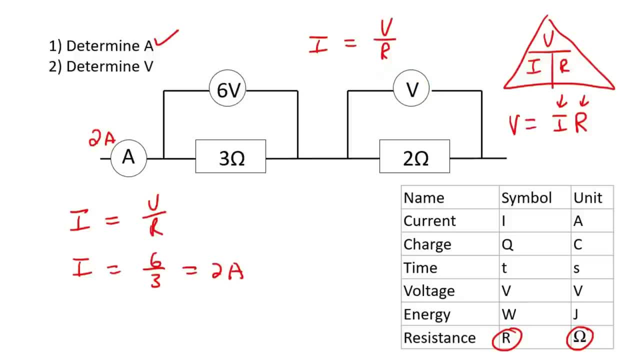 we need to use, because we're looking at this volt meter, which is connected across this resistor. so we know what the resistance is, but we don't know what the current is. we don't have a current value. however, we have learned that when you are in series, when the electricity flows like that, 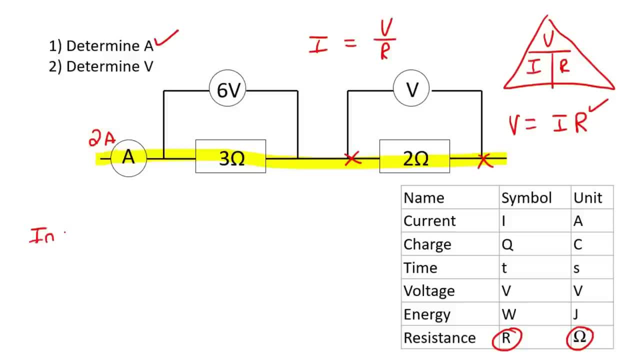 then the current remains constant. remember, in series, current remains constant. so that means then that this is also going to be the same as this current value over here, because if you have two amps over here, then that two amps is going to flow all the way through. so now we know the current as two, we know that the 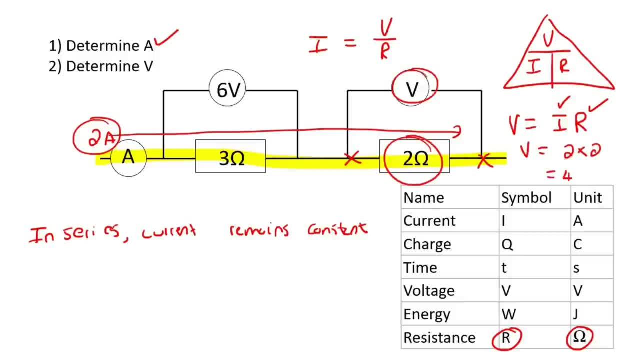 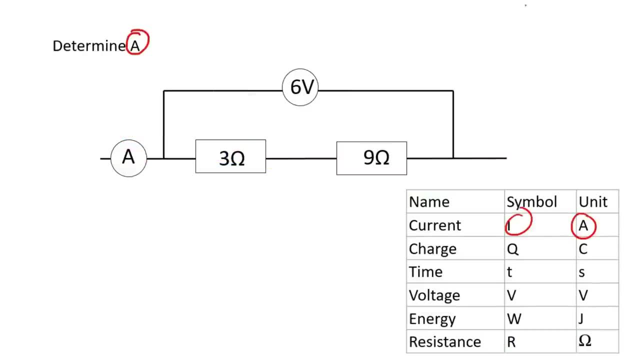 resistance value is two, and so this volt meter will be four volts. four volts, all right. so here's one last thing we need to consider now. the result i have given to me is what we are going to actually calculate over here. probably one cow, 14 volts V. that's just a short figure, something like that. 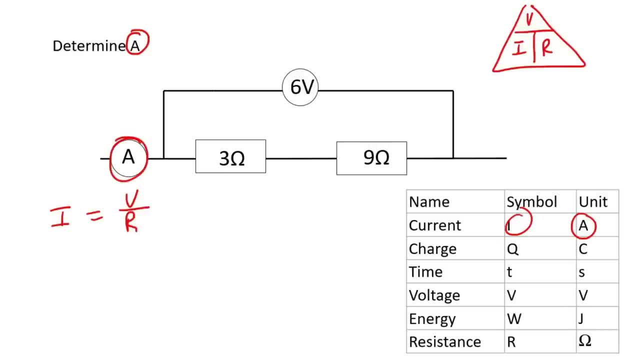 we're going to use that to假 state. let's say that mol, over here that's a mol topics, and we're going to use the right of gn focused. We want to multiply that number by expanding it essentially and the one difference that it makes. well, let's say I did a cotton test and we're supposed to determine the polеннойて. 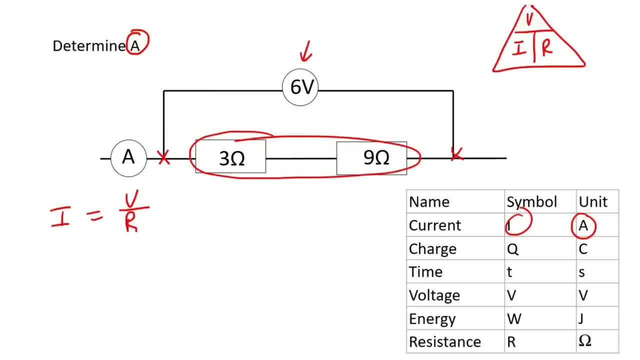 is both of these. so if you want to use that voltage of six, then you need to use these resistors. now remember: these resistors are in series and we've learned in previous lessons that when resistors are in series you just add them together, so you just say three plus nine. you don't have to. 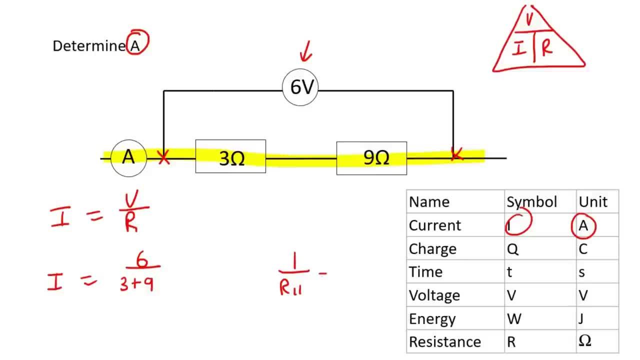 use that weird r parallel um is equal to one over r1 plus one. that's only when they're in parallel, which we'll look at a little bit later, but in series you just add them together, okay, so that's going to give us six divided by 12 and that's going to give us 0.5 amps. so here's our first. 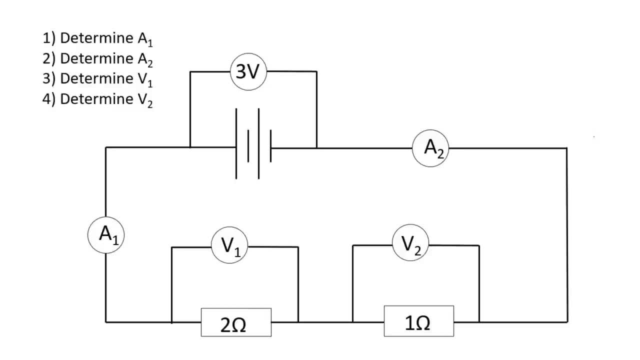 proper circuit um example now. so the first question says: calculate a1. okay, so from our formulas, which we have over there, um, they want us to calculate current. so we know that current is equal to voltage over resistance. now you've got to be careful with which voltage you actually go and use. so, or you got to be careful with which voltage. 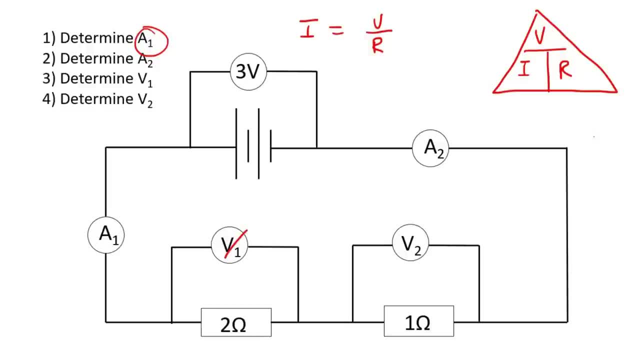 and which resistor you use. they have to go together. so we don't know what this voltage is. we don't know what this voltage is, but we do know what this voltage is. now. this is the battery voltage. okay, that is your battery. so if you use the battery voltage, okay then which resistors do? 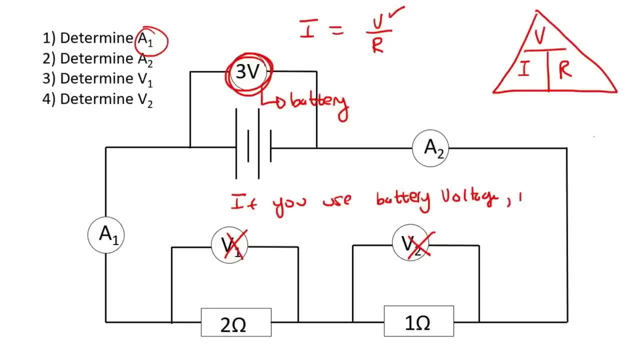 we need to use. well, the battery is everything. so then you will use all resistors. so we need to go add up all of the resistors. but we need to be careful. are we in parallel or are we in series? because in parallel you add the resistors differently to if you are in series. remember that in series you just add all of them. 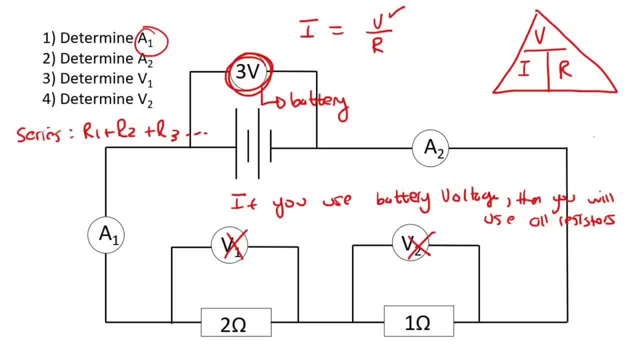 together. so you just keep adding all of the resistors, but then, in parallel, you've got that weird formula that does something like this. okay, so we need to go check: are we in series or in parallel? some of you can identify it immediately, but if those of you that are struggling, let me 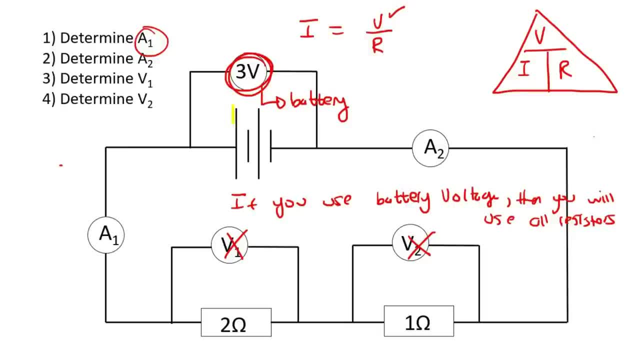 quickly try explain so we know that the electricity starts over here and then it flows through the circuit like that. so can you see that the path never changed. we didn't go, we didn't split up, like we've seen in previous lessons. so this is a uh series circuit. so the total uh resistance. 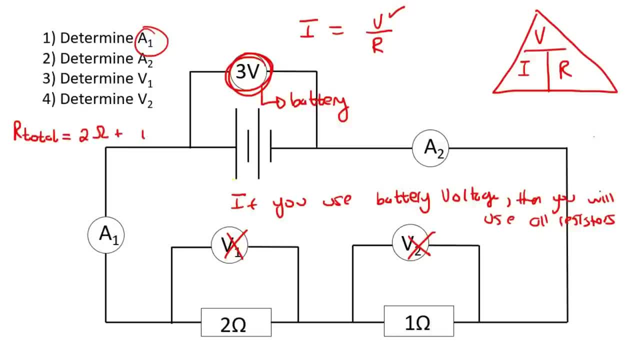 would be, um, the two ohm plus the one ohm, and that would give you three ohms. so that is our total resistance. so we know the voltage and we know the resistance. so we can now say three divided by three and that'll give us one amp. so that is the current flowing in the whole circuit, because we used 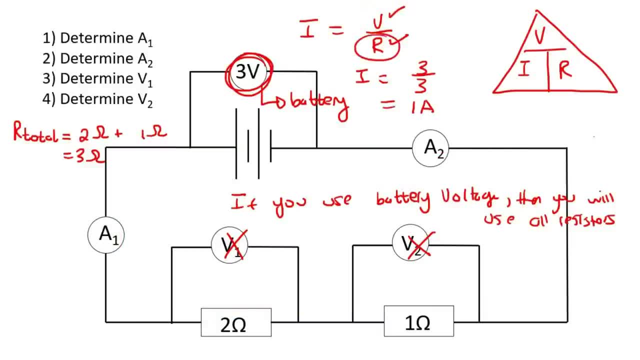 all of the voltages, which is the battery, and we used all of the resistors and so that is going to give us the current in the whole main part of the circuit. so that means the current here will be one amp and over here one amp and everywhere one amp. it will be one amp of the year, one amp of the year. 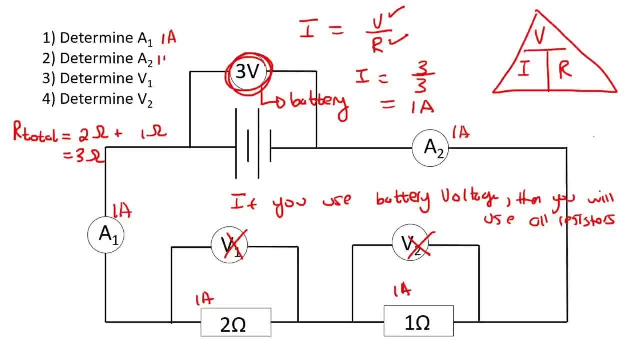 everywhere the current will be one amp. so here we can say one amp. here we can say one amp, because we've learned that current in series remains constant. the next question asks us to calculate v1 over here. so v1 is connected across this resistor. so when you use the formula for voltage, which is v, 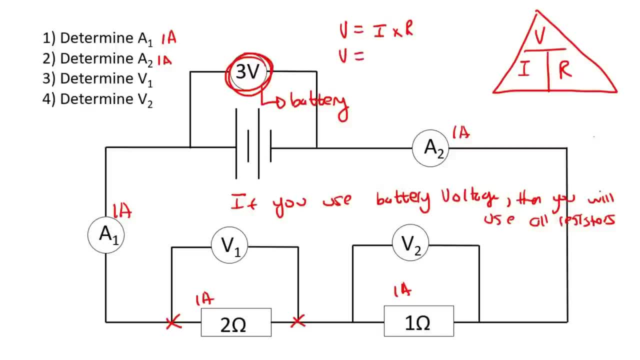 equals to i times r? um. you're going to use the currents that goes through that one, which is the one amp, because the current is the same everywhere, and then you're only going to use that resistance value, because this volt meter is only connected across that resistor and that would give you 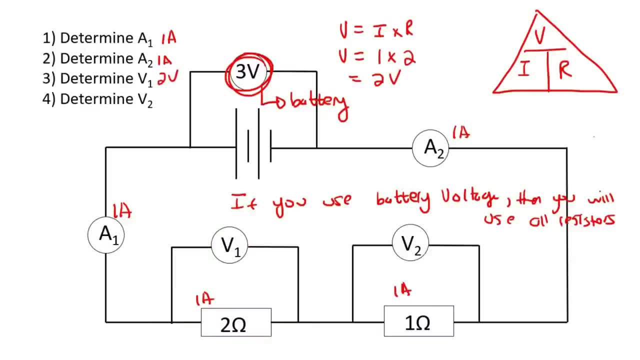 two volts. okay, so that's two volts. the last question says determine v2, which is this one over here. so check this out. we've got the current and we've got the resistance for that particular volt meter, which is only connected across there, and so you could say v. 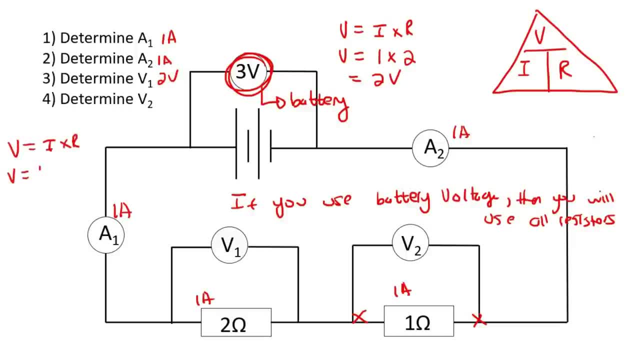 is equal to i times r, and so v is equal to one times one, which is one volt. for those of you that are curious, notice how these two volt meters, when you add them together, two plus one, gives you the battery voltage. that is something we have looked at in previous lessons. um, for those of you that 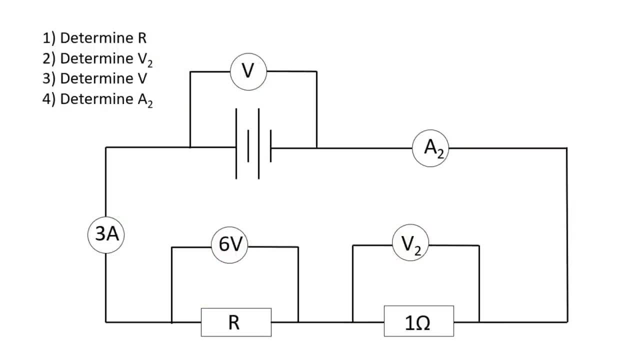 are interested about that. okay, let's go to our next example. so here's our next example. so the first question says: calculate r. okay, so from our formulas we've got this over here. so if you want to calculate r, well, that is going to be: r is equal to v over i. so if you look over here, r. 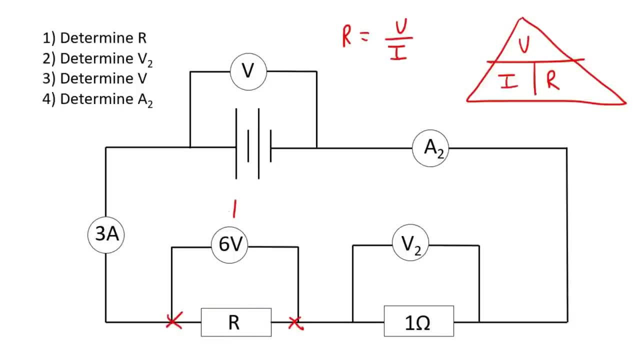 is connected between this volt meter, so we're definitely going to use that six volts over there, and so to calculate r, we going to use this. in this case, we're going to use the voltage. okay, now we need a current. they've told us that the current here is three amps. now, because the 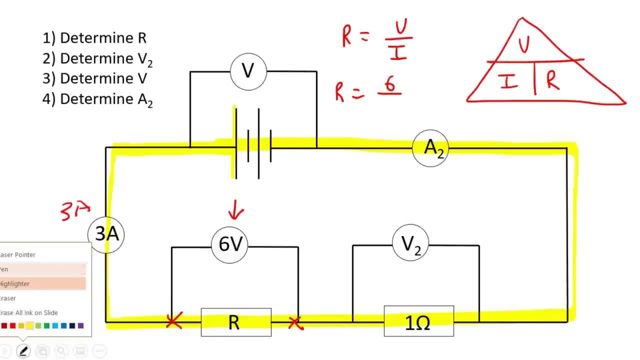 circuit is in series. have a look here. see that it's in series. well, what that means is that the current going through this resistor is also three amps. so we have the current and so, and so then, if we had to go work this out, you're going to end up with two ohms. remember that. 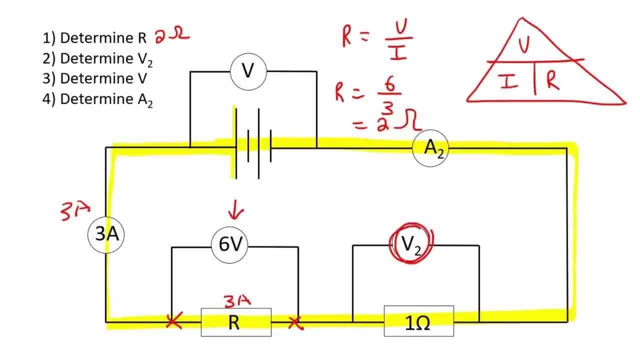 is the Okay, so V2 is over here. So we know from these formulas that to calculate voltage you have I times R. Now we know that this voltmeter is connected over here, So it's connected across this resistor. So that's the resistance that we would use. 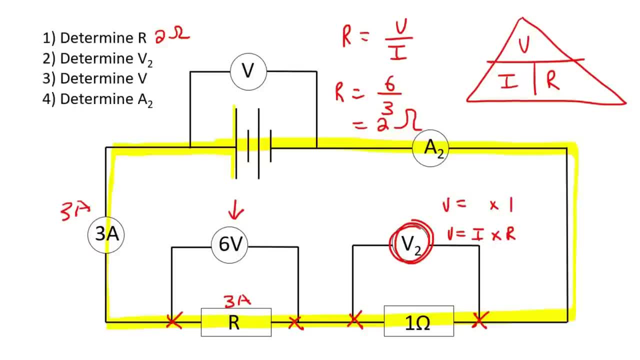 So we've got the resistance as 1.. Now we just need the current that is going through this resistor. So we know that the current in the main circuit is 3 amps. So that means that that current all the way through is going to be 3 amps. 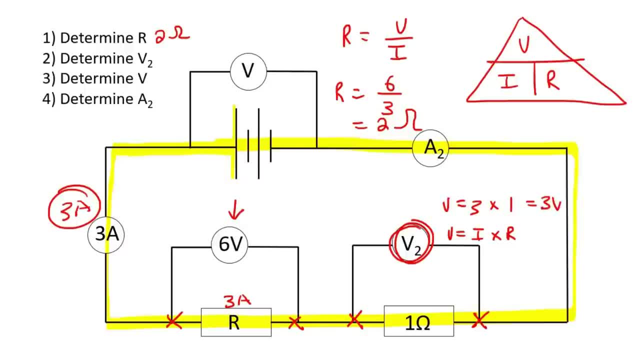 So we can just say 3 over there And if you have to calculate that you're going to end up with 3 volts. So V2 would be 3 volts, So let's just fill that in there as 3 volts. The next question says calculate V. 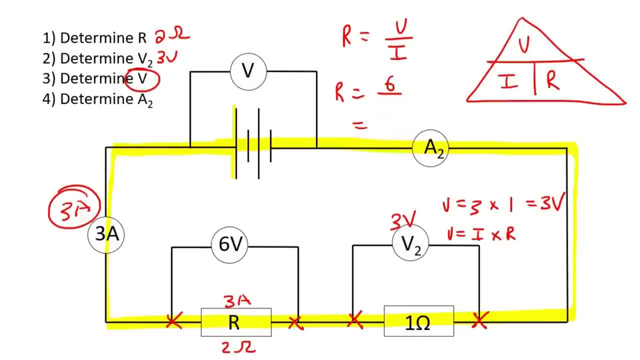 So there are a couple of ways that you could do this one. One of the ways is to remember the formula that I've showed you in previous videos And I've shown you in previous lessons, which says that the voltage of a battery is equal to the sum of all of the voltages in series plus the parallel branches. 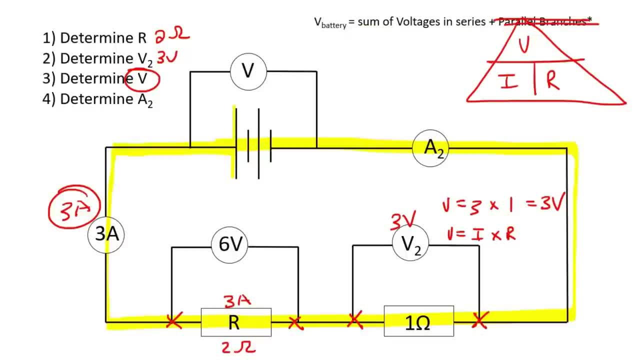 Now we don't have any parallel branches so we can just ignore that. So the voltage of a battery is the sum of all of the voltages in series. That would be 6 volts plus 3 volts. So that would be 6 volts plus 3 volts, which is 9 volts. 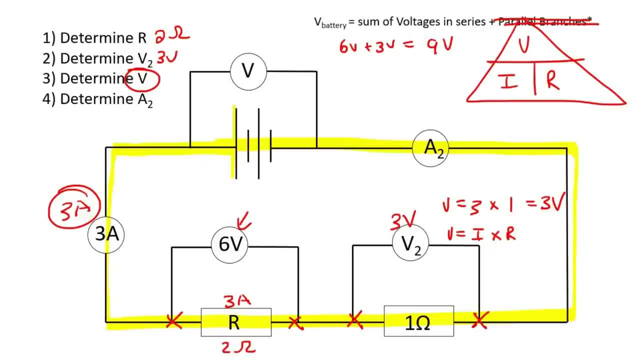 That's one way to do it. The other way you could do this question is: you could use a formula So you could say voltage is equal. So you could say: voltage is equal to current multiplied by resistance. Now, if you are looking for the battery's voltage, remember what I showed you in the previous example. 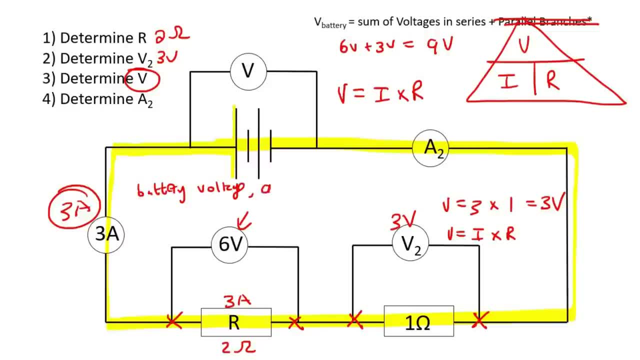 If you are using the battery voltage, then you must use all the resistors. Then you must use all of the resistors And you must use the current that is part of the main circuit. So that means you would use this resistor over here, which is 2 ohms. 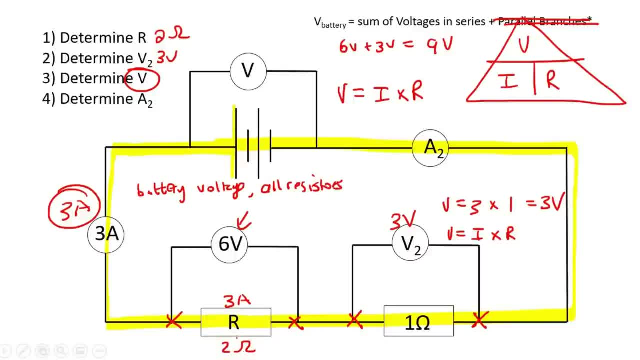 And you would use this resistor over here, which is 1 ohm, And because they're in series, you would plus them together. So the total resistance Is going to be 2 plus 1, which is 3 ohms. 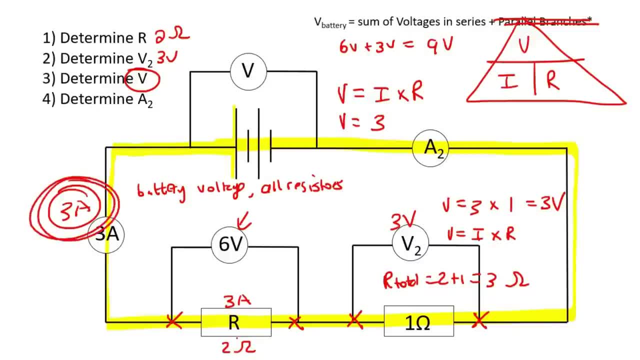 So then the voltage would be the total current Multiplied by the total resistance, And that would give you 9 volts. So it's the same exact answer. The last question for this particular example says determine A2.. So A2 and A1, or this one- are going to be exactly the same. 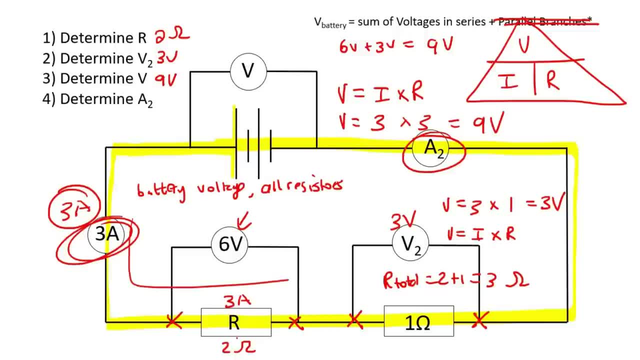 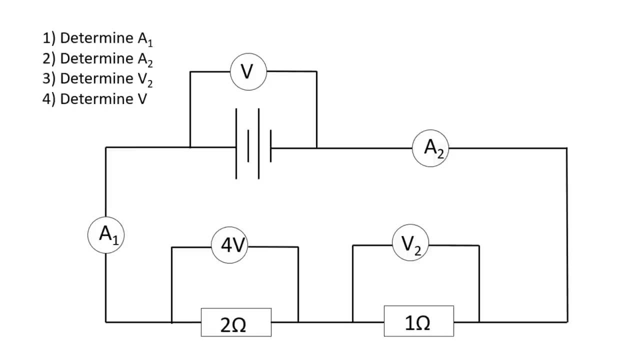 Because this circuit is in series And so all of the current stays the same, And so that will simply be 3 amps. So here's our next example. So this one says: the first question says: determine A1.. Okay, So from our formulas, which from our triangle of formulas like this: 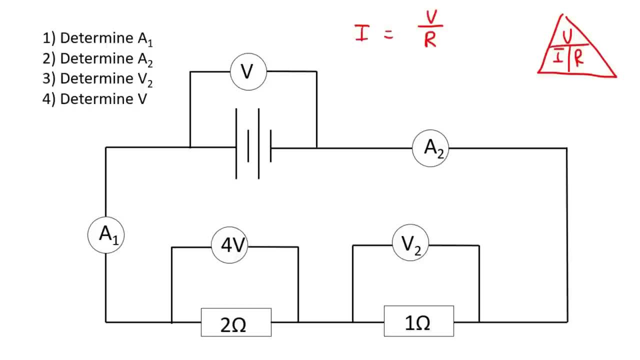 To work out current, you need to know voltage over resistance. Now, what voltage do we use? Well, we don't have this voltage. We don't have this voltage, But we do have this voltage. So if you are going to use this voltage, 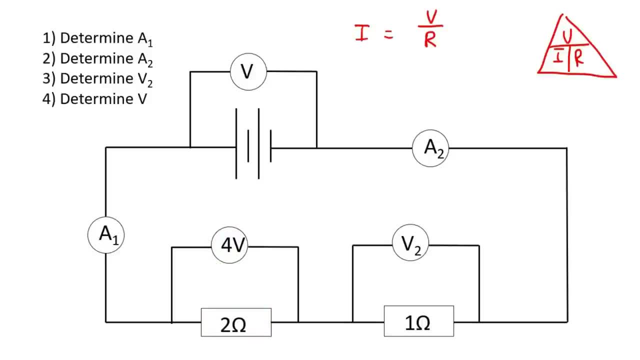 Then you need to use this resistor Because this voltage is connected only across that resistor. So you're going to say: I is equal to 4 over 2, which is 2 amps. But now some of you might say, yeah, but Kevin, doesn't that mean that the current going through this resistor is 2 amps? 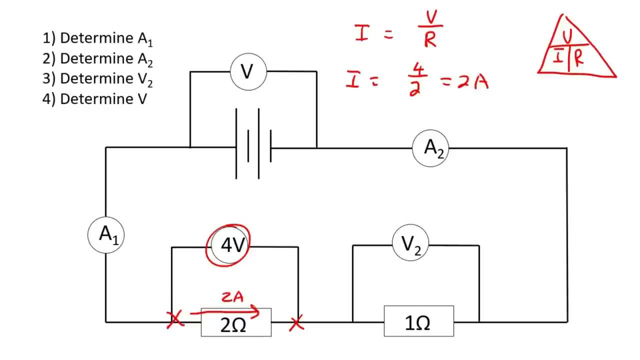 Yes, that is correct, But we know that current in series is the same everywhere. So if we've just worked out the current over here, Well then that is also the current over here, Over here, over here, everywhere, Because current in series stays the same. 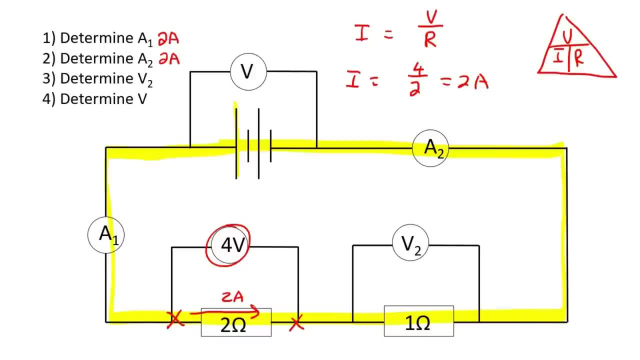 So we can say 2 amps over here and 2 amps over here. The next question says calculate V2, which is over here. So to calculate voltage you need to say current multiplied by resistance. Now we know the current because current stays the same everywhere. 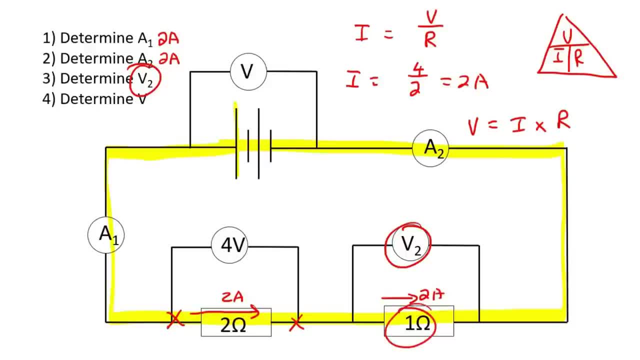 And so we also know the resistance that is connected between that voltmeter, And so we can just say 2 multiplied by 1. And that's going to give you 2 volts. OK, so we can say 2 volts. The last one for this particular question says determine: 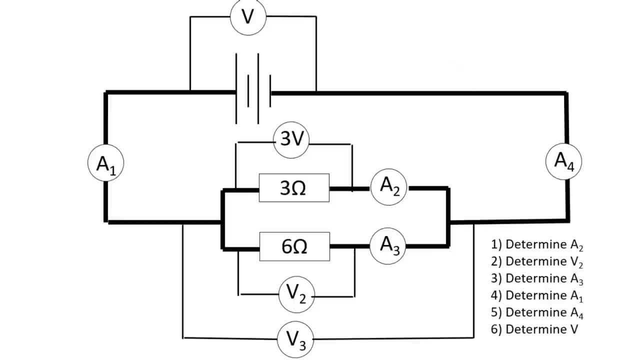 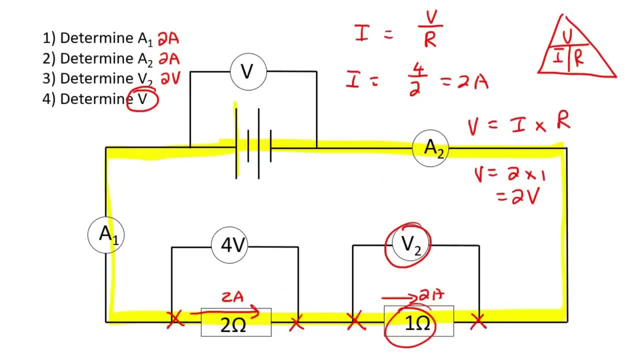 And, by the way, we're going to get to a whole bunch of parallel examples coming up now And we're even going to do an example that has a parallel and part that's in series- OK, and then we would be done. So it says: calculate the voltage. 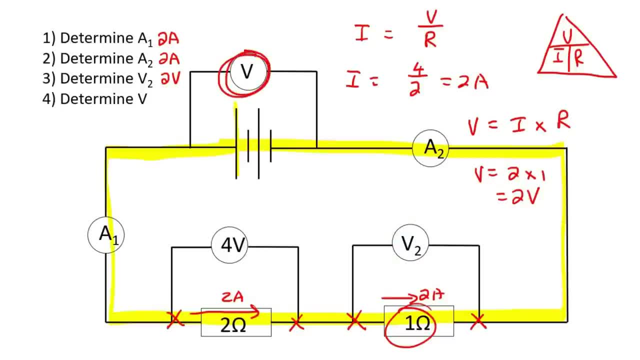 Now, once again, there are two ways to do this: To calculate the battery voltage. So you could either use this formula again- We don't have any parallel parts, So you could just say that the voltage of the battery is equal to the sum of all of the voltages in series. 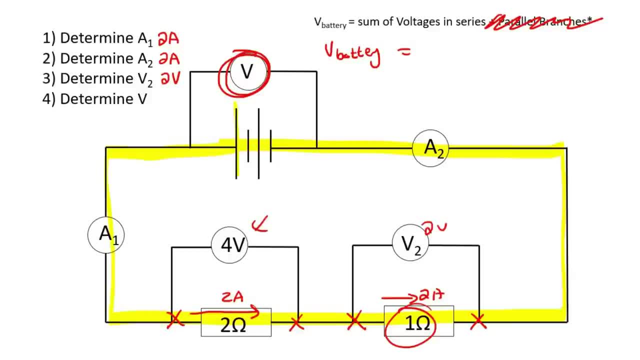 That would be 4 plus this one which was 2 volts. So that would be 4 plus 2, which is 6 volts. Your other option is to use the voltage formula, which is: V equals to I times R, And so your current in the main circuit. 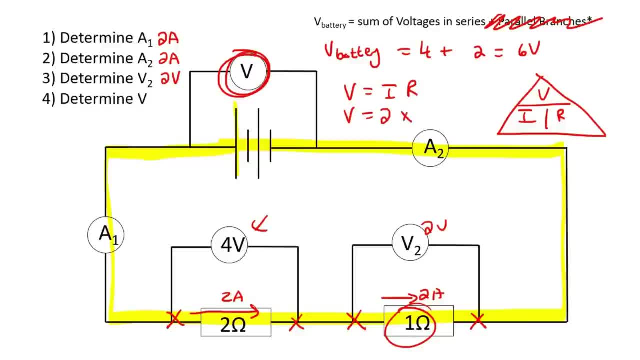 Is 2 amps, which we already found, And then you would have to use the total resistance. because you're using the battery, You have to use all of the resistors. So the total resistance Would be 2 plus 1, which is 3.. 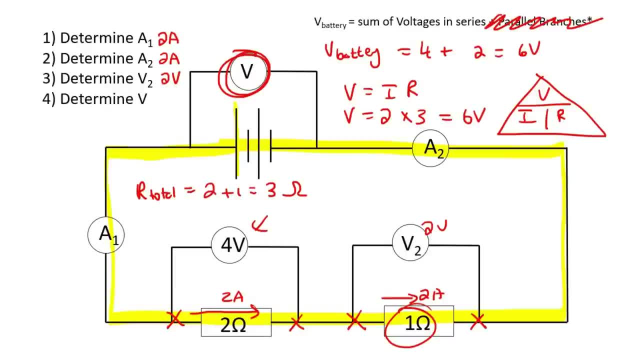 So you could say 3 and that would give you 6 volts. So whether you use that formula or that formula, you're going to get 6 volts for the battery. Some teachers might call the battery, the voltage of the battery, the EMF. 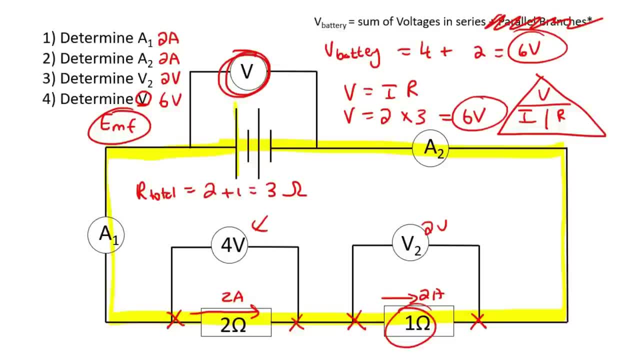 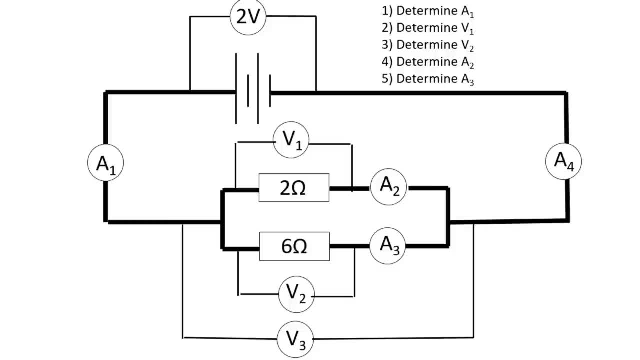 OK, I haven't mentioned that. I actually forgot. I haven't mentioned that at all. So yeah, EMF is another name for the voltage of the battery. OK, so here's an example where we're going to be having a parallel scenario. 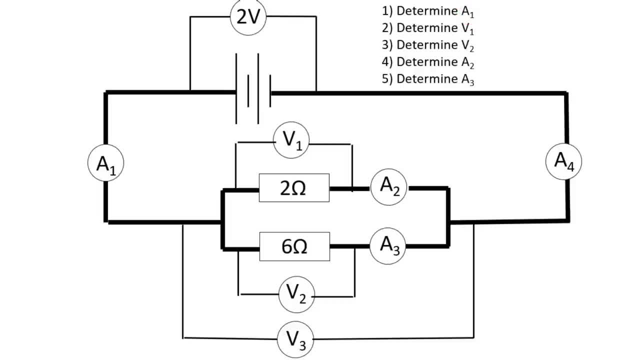 OK. so the first question says: calculate A1.. So A is a current right. So that's I. So to calculate current, you say I equals to V over R. So we need a voltage. Now there's no voltage here, no voltage here, no voltage here. 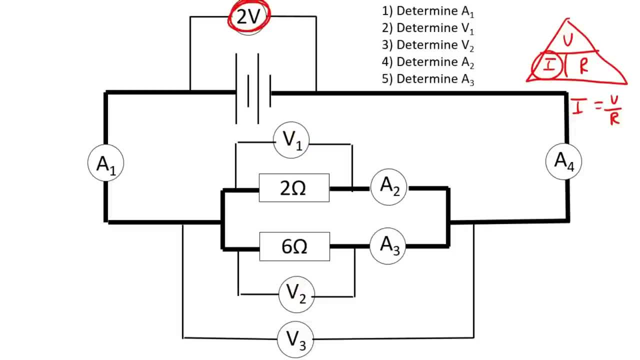 However, we do know the battery's voltage is 2.. OK, So if we use the voltage of the battery, then we need to use all of the resistors. Remember that if you use battery voltage, then use all resistors, But you need to understand if you are in series or in parallel, or sometimes, as we'll see, 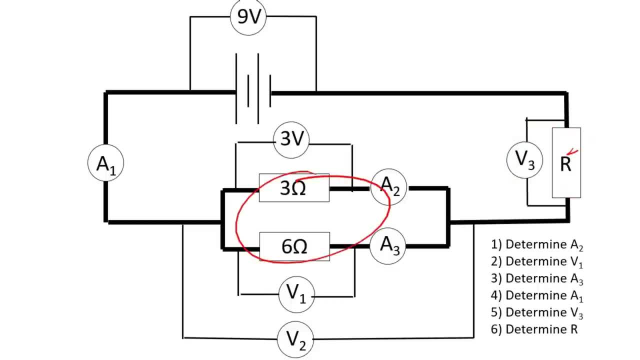 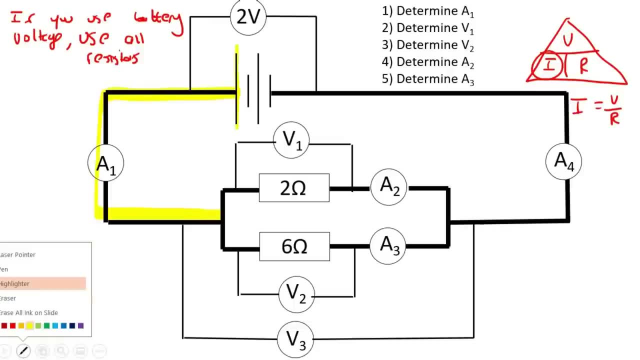 later you're going to have series and parallel, or let's rather say parallel and series. So if we go look at the circuit, we can see that it is in parallel because some of the current is going to go this way and some of the current is going to go this way. 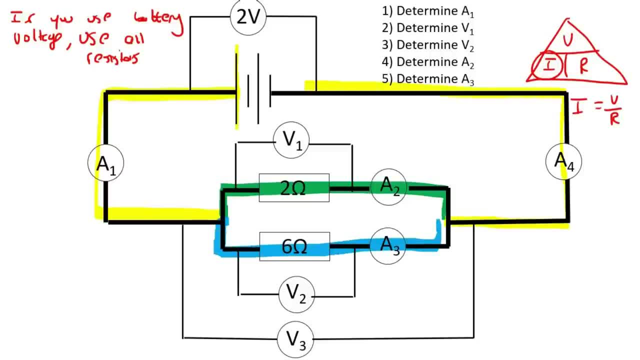 And then all of the current will resume like that. So this part is in parallel. Do we have any other resistors? No, we only have those two. So we need to go combine them in parallel. So the way that you do that is you say one over R, parallel is equal to one over two plus. 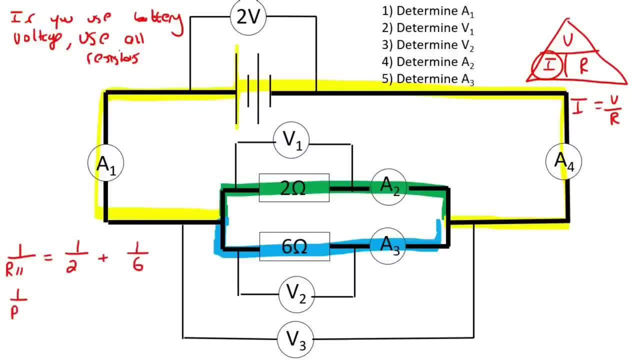 one over six, Then you're going to go type that on your calculator And that'll give you two over three. Then you're going to flip both of these upside down So you end up with R. parallel is equal to three over two, which is the same as one point. 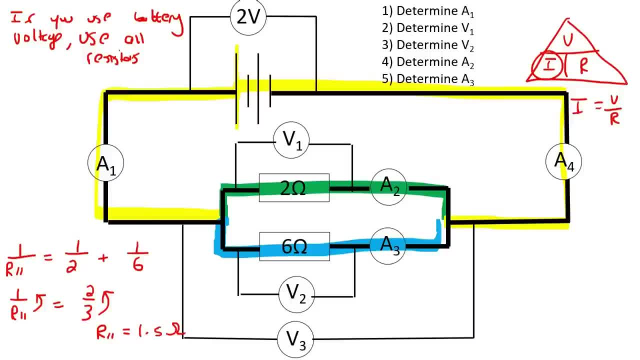 five ohms. one point five ohms. OK, So now we know the voltage We're going to use that and we know the total resistance, so we can go work out the current. so we can say two divided by one point five and two, three. 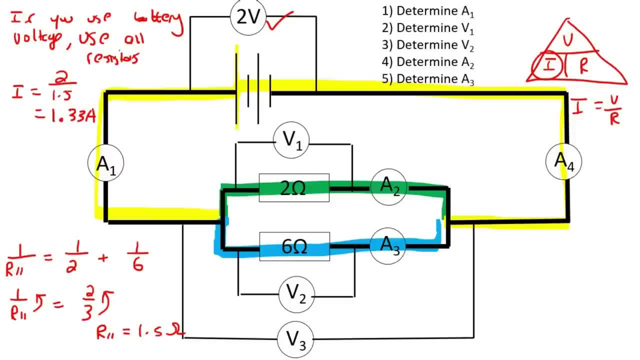 That would give you one point three, three amps. So now we can use that current for the rest of the lesson. One point three, three amps. And let's just fill it in over here as well, OK, The next question says calculate V1.. 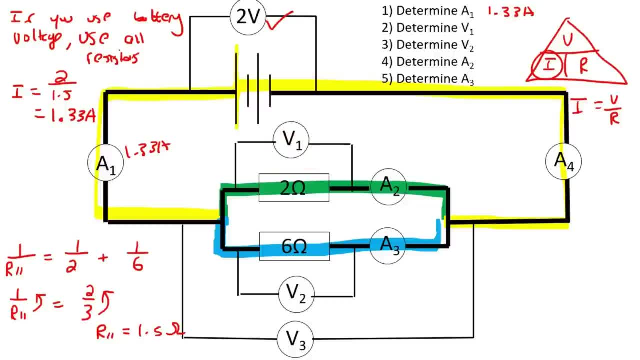 Now V1 is over here. OK, So now- this is important- We know the resistance for V1.. V1 is connected across this resistor. So we know the resistance, but we don't have the current. You cannot say That this current is the same as this current, because this part is in series. 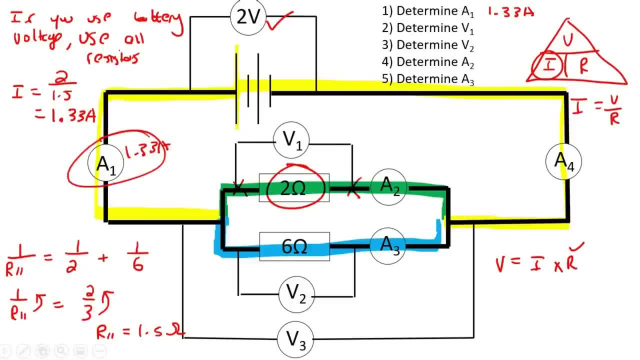 This part is in a different pathway, So the current is not the same, So this formula actually won't work. What we're rather going to do is remember this formula, Which tells us that the voltage of the battery is equal to the sum of all of the voltage in series plus the parallel branches. 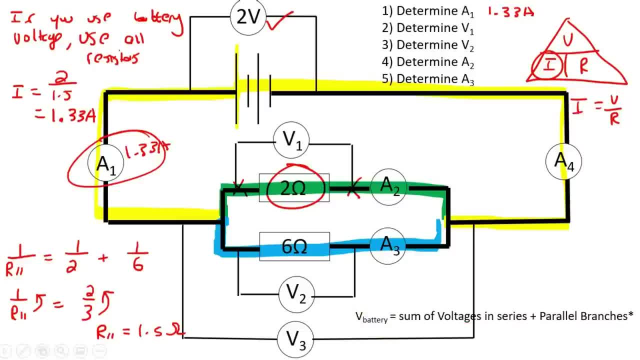 Now this circuit doesn't have any series resistors, So there's no voltages in series, So we can ignore that. So then we can just say that the battery's voltage is the same as the total parallel- The branches in parallel. So the voltage of the battery is two. 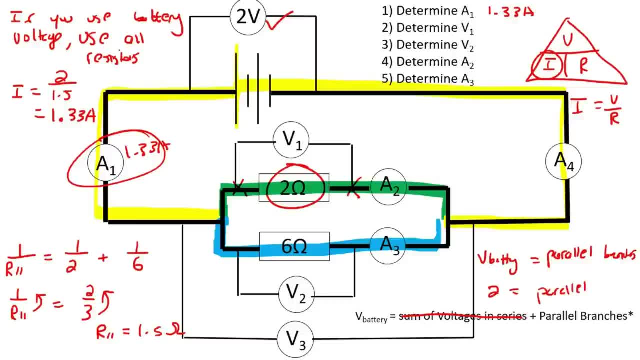 So we can say two, And so the parallel branches are each going to be two. So that means that this one is two, This one is two, And this one is also going to be two volts. So there, we've got the voltage in parallel. 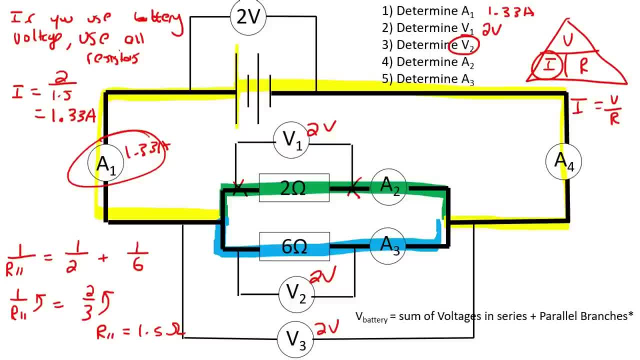 There, we've got V1 as two volts. Now the next question says: what is V2?? So V2 is also two volts. We've got that one. The next one says: what is A2?? Okay, so A2 is over here. 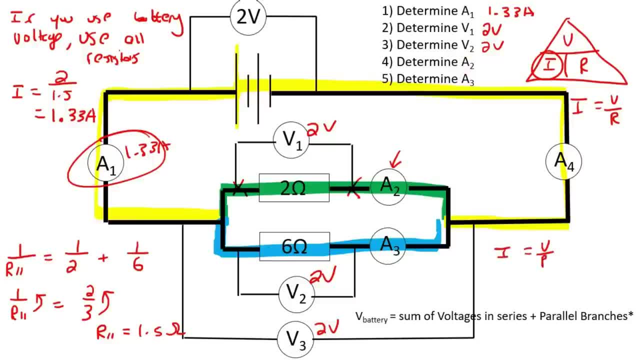 So that's a current. So current is equal to voltage over resistance. Now you've got to be careful. This current ammeter is connected on the green pathway. It's only the green pathway, So you need to look at on the green pathway. 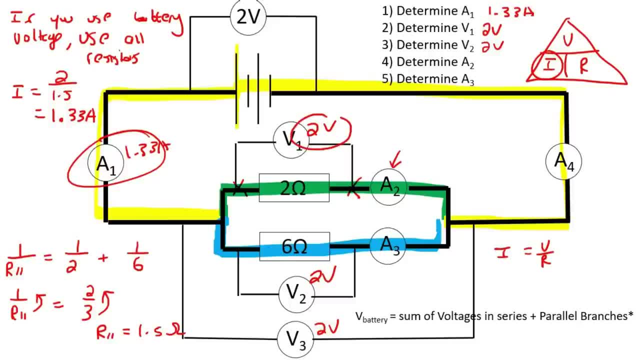 So voltages and resistors on the green pathway. So here we've got a voltage And it's connected across this resistor, So we can use those two. So we could say two divided by two And that'll be one amp. Okay, so this is one amp. 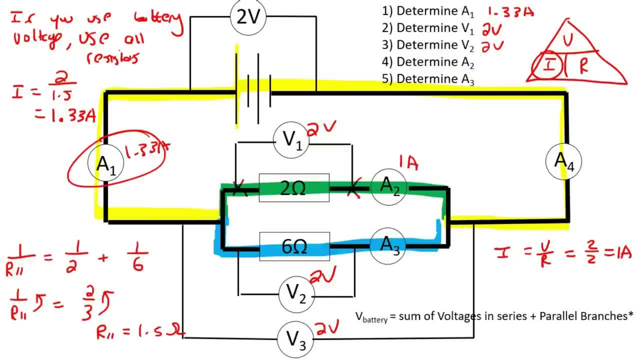 The next one says: calculate A2.. Oh no, that's the one we've just done. The next one says calculate A3.. So that's this one. Now, there are multiple ways that you could do this. one You could either use: I equals to V over R. 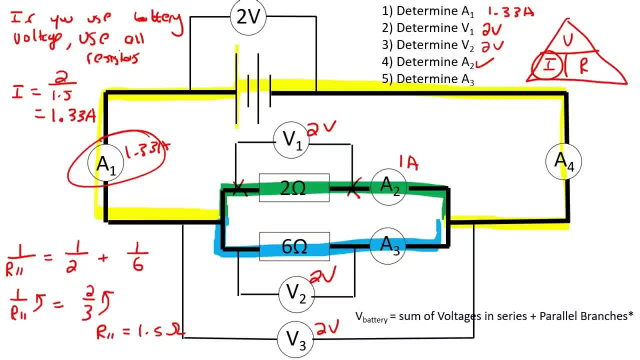 And you could use the six and the two. Okay, Let's just try that. So I is equal to V over R, And so the voltage is two, And that two is connected across the six ohm resistor And that'll be 0.33 amps. 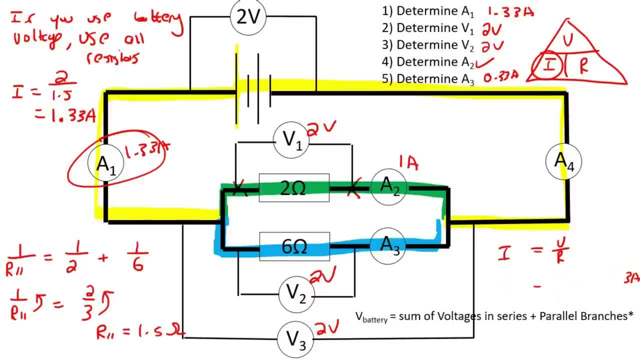 Okay, That's one way to do it. The other way is to remember what we said in previous lessons, like this: So we learned that the sum of currents in parallel is equal to the current in the main circuit. So the current in the main circuit is A1.. 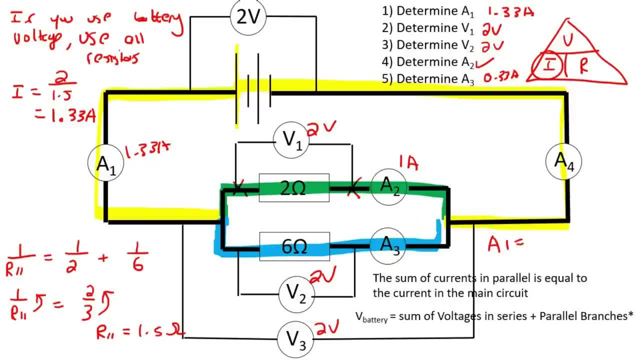 So that'll be the same as the sum of the currents in parallel. So that's A2 plus A3. So that would be: 1.33 is equal to A2, which is 1 plus A3. Now if you had to go calculate A3, you would end up with 0.33 amps. 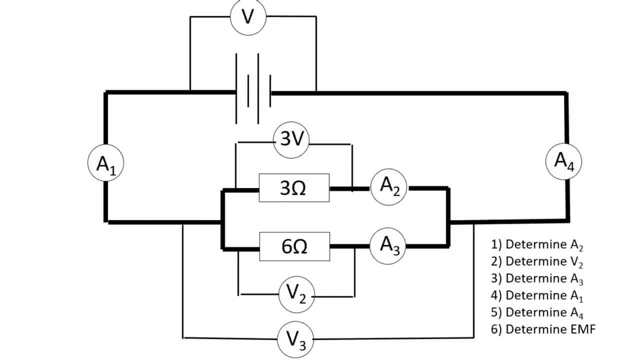 Which is exactly what we got over there. So we only have two more examples now. All right, So well done for making it this far. We've just got this example, which is another parallel one, And then we've got one over here which has a parallel or a series and a parallel combined. 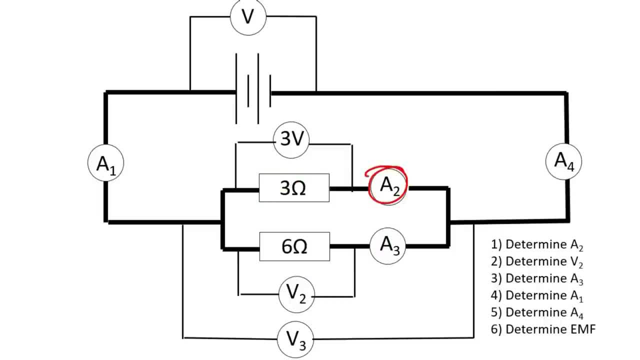 So the first question here says Calculate A2.. Okay, So if we look at the formulas, we know that to calculate current we could try using V over R. So let's see what voltmeters we have. Well, A2, if we look carefully, we know that current flows like this: 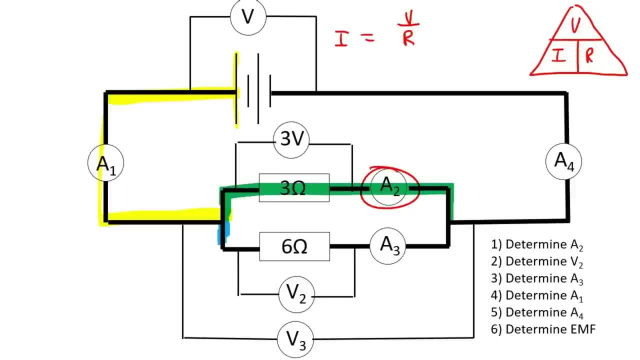 Then, when it gets here, some of it would go this way and the rest would go this way. It would then combine and go like that. So if you're calculating the current that's going through A2. Well then you need to be only looking at this branch over here. 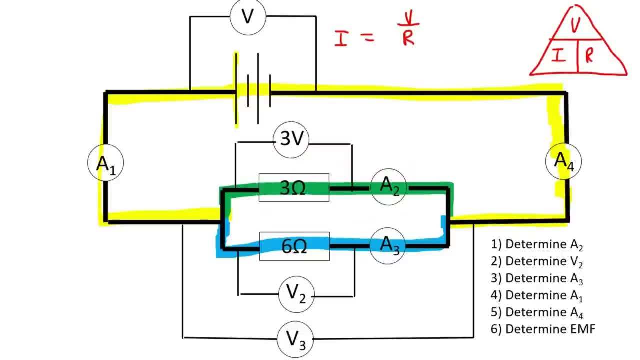 So if you look at the voltages in that branch, we've got this one over here And that is connected to this resistor, So those are going to be perfect. So we can say 3 divided by 3, which is 1 amp. 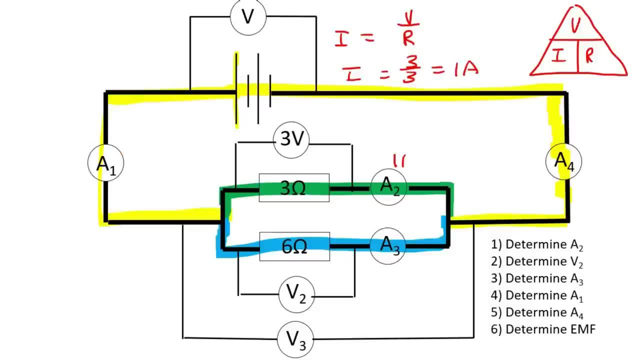 So that doesn't mean this is 1 amp. No, That means this is 1 amp. Okay. So that's done. Determine V2.. Now V2 is over here. We know that in parallel, all voltages Are the same. 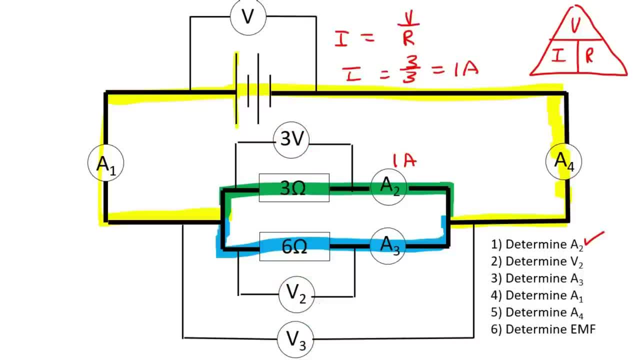 All voltages are the same in parallel. So V2 is also going to be 3 volts Because this path is 3 volts. So this path would be 3 volts And this would also be 3 volts. The next question says calculate A3.. 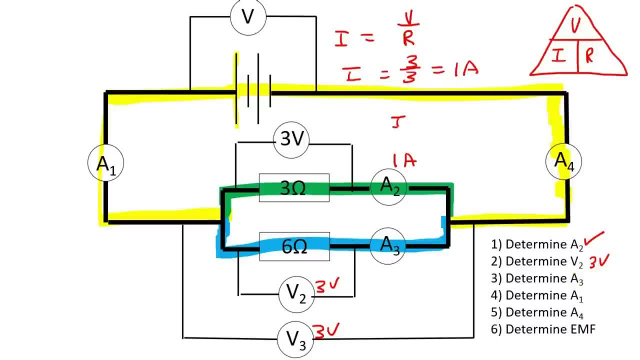 Now A3 is over here, So we could use. I equals to V over R, Where the voltage in that pathway is 3 volts And the resistance in that pathway is 6. And so we could get 0. 5 Amps. 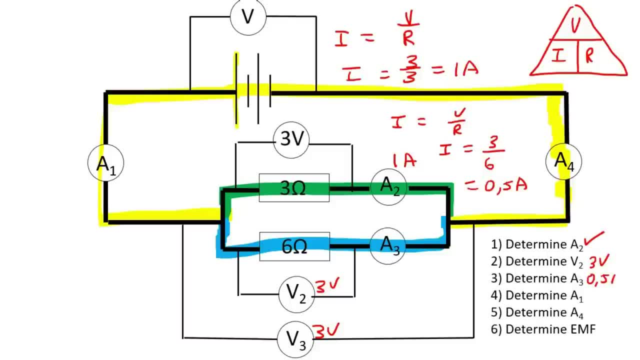 So 0., 5 Amps. The next question says: calculate A1. Now there's. Now. A1 is here. Now there's multiple ways of doing this, But one of the easiest ways is to remember Is that the sum of currents in parallel is equal to the current in the main circuit. 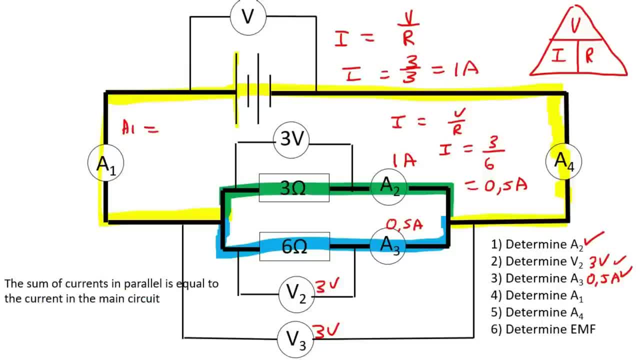 So that means that A1., Which is part of the main circuit, Is equal to A2 plus A3. And so, And so A1 is going to be equal to 1 plus 0,5, because that's A3, and so that's going to give us 1,5 amps. 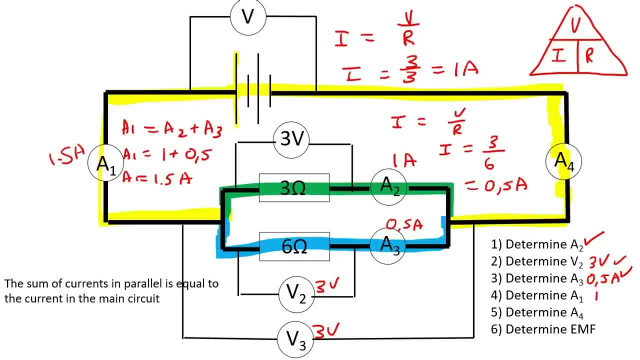 So A1 will be 1.5 amps, 1.5.. Now the next question says: calculate A4, but now A1 and A4 are going to be the same because they are both in series and so that is going to be 1.5 amps. 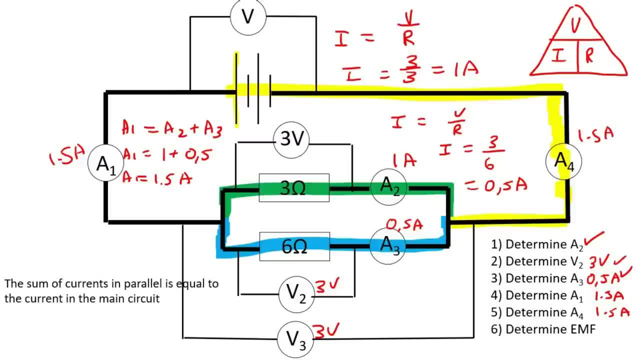 Now the last question for this particular question says the EMF. Now, remember, EMF is something I introduced a few minutes ago in one of the previous examples- is actually just the voltage of the battery. That's what EMF means. 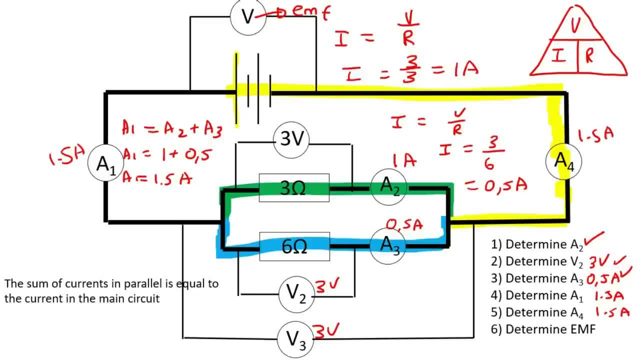 So there's multiple ways to do this question now. One of them is to use the formula for voltage, which is V equals to. well, let me show you the easy way first. The easiest way would be to remember this formula over here, which tells us that the voltage of the battery is equal to all of the voltages in series. 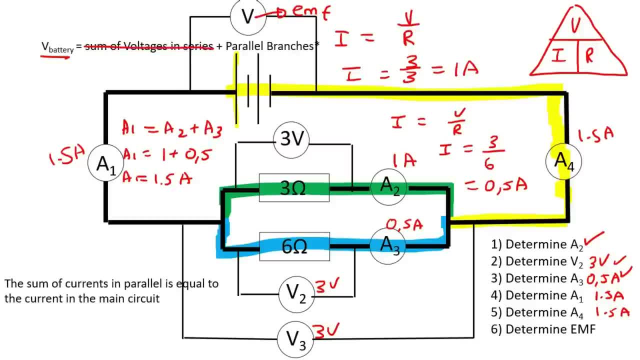 We don't have any voltages in series, and then it's equal to plus any of the parallel branches. So we can just say that the voltage of the battery is going to be equal to the parallel branches, And so we know that the parallel branches are 3 volts, 3 volts and 3 volts. 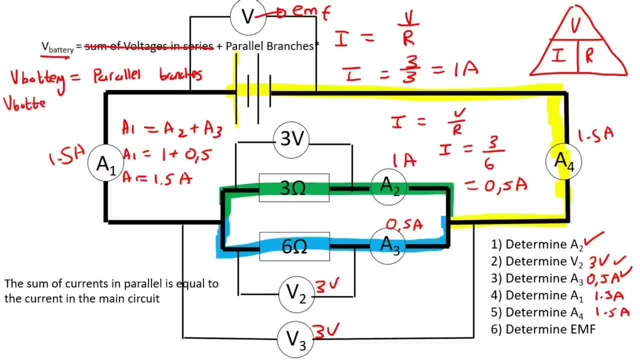 So we can just say that the voltage of the battery is 3 volts. Okay, now the other way you could have done this- it's a little bit longer, but it would work and I want to show you so you can just see that it does actually work- is to use the formula for voltage. 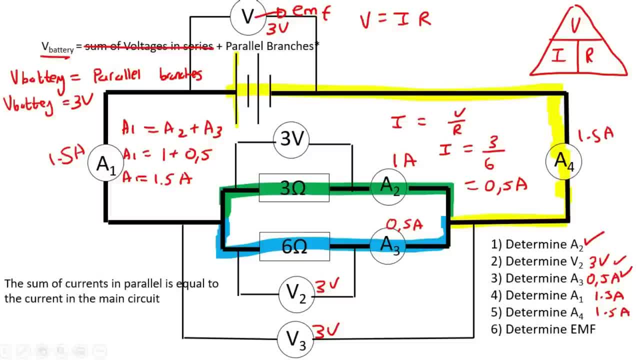 Now, because you are looking for the battery voltage, then you need to use the total resistance in the circuit and the total current in the main circuit. So we already know the current in the main circuit is 1.5.. Okay, so we could say 1.5.. 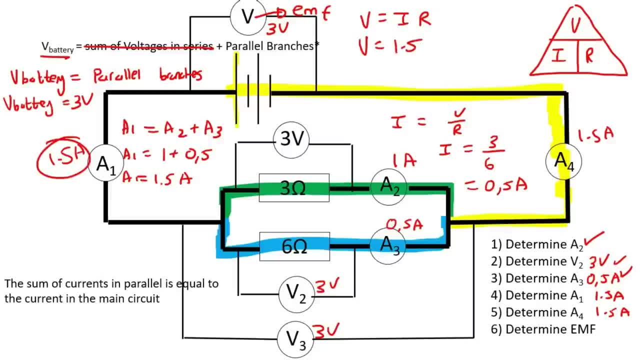 Now we need to go get the total resistance of the whole circuit, which is only these two, but they are in parallel. So you're going to say 1 over R. parallel is equal to 1 over 3 plus 1 over 6.. 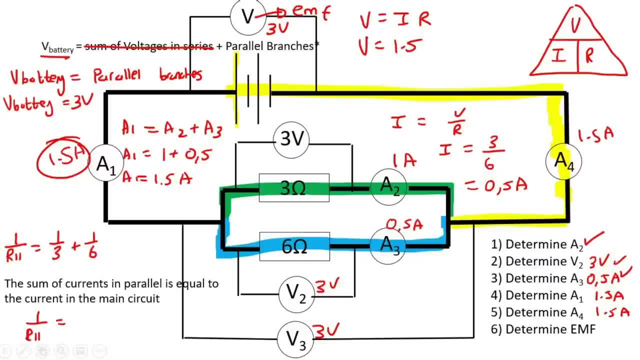 And so 1 over R parallel is going to give you. so you just say 1 over 3 plus 1 over 6 on your calculator and that'll be 1 over 2.. Then what you do is you switch everything around so it becomes: R parallel is equal to 2 over 1, which is actually just 2 ohms. 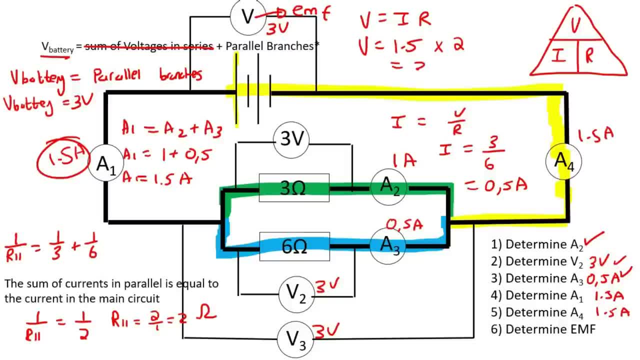 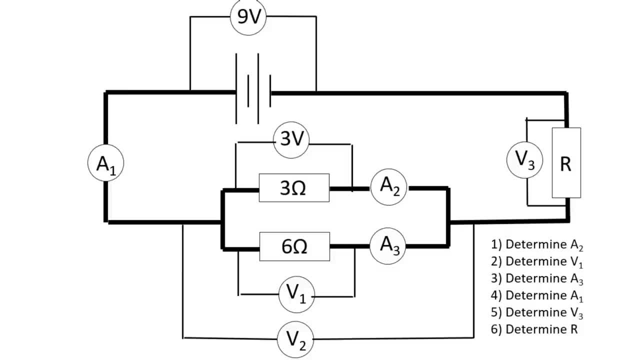 So then you could say: 1.5 multiplied by 2, and that would give you 3 volts. Same answer, So we can say: they're 3 volts. Let's do one more example. So this one says: now, this one's pretty awesome, because we've got a parallel part where the current's going to go there and then it carries on in series again over there. 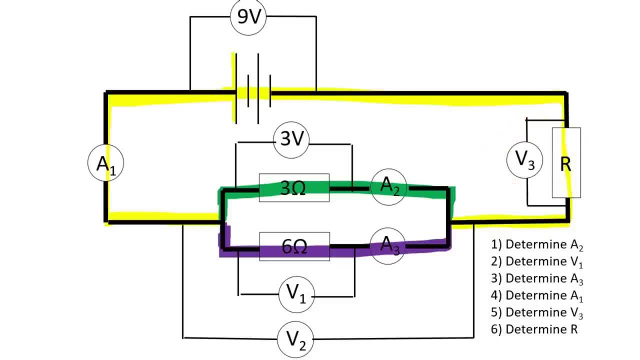 So we've got a bit of series and parallel with a device in series there. So the first question says: calculate A2.. Now A2 is over here, So that's not part of the main circuit. So if we look at these formulas we know that current is equal to voltage over resistance. 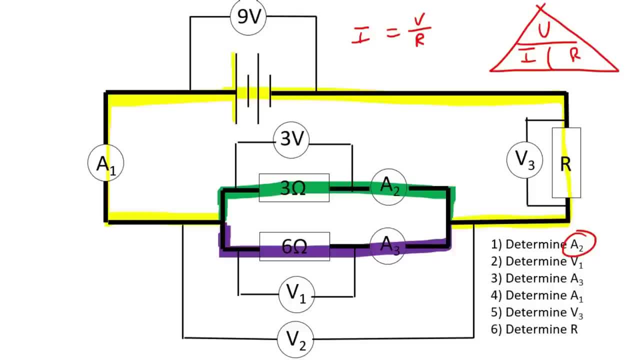 But now this current is part of the green pathway So you can use this 3 volt which is connected to this 3 ohm. You see it's connected across this 3 ohm over here. So you could say I is equal to 3 over 3, which is 1 amp. 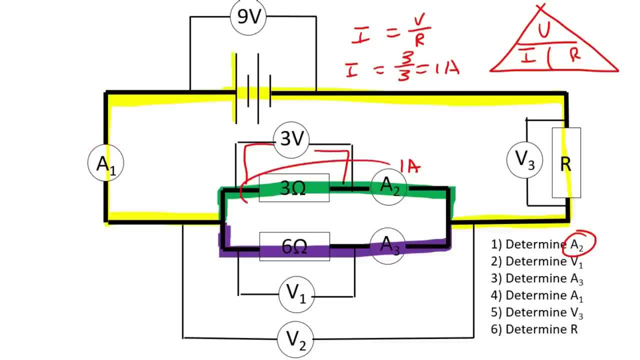 That does not mean that this is 1 amp. It only means that it's 1 amp over there. Okay, So we've got that one, Fantastic. The next one says: calculate V1.. Now V1 is over here. Now we know that parallel voltages, the pathways, have the same voltage. 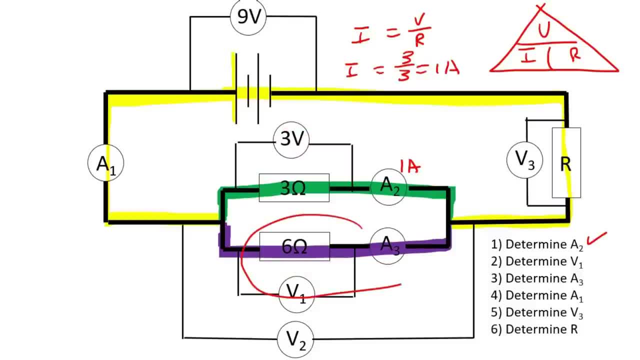 So this pathway has a voltage of 3, and that means this pathway would also have a voltage of 3.. So V1 would be 3 volts. This question says: calculate A3.. Okay, So A3, we could use. I equals to V over R and we know the resistance. 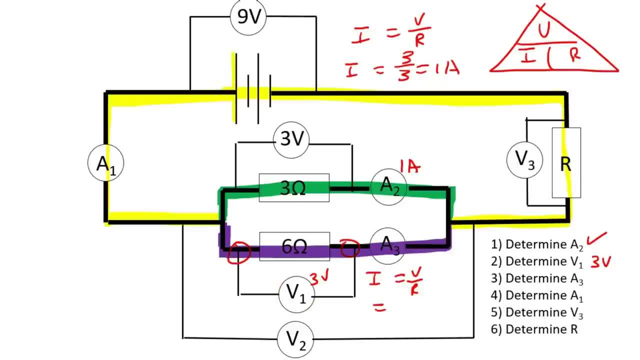 And we know the voltage connected across that resistance or that resistor. So we could say 3 divided by 6, which is 0,5 amps, So 0,5 amps. The next one says: calculate A1. Now we know that the sum of the currents in parallel is equal to the current in the main circuit. 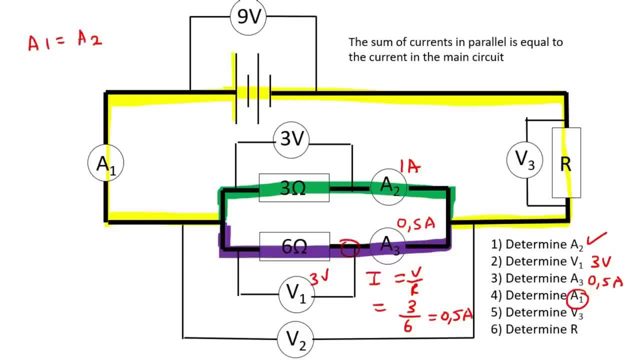 So that means that A1 is equal to the sum of all of the currents in parallel, which is A2 plus A3. And so A1 is going to be 1 plus 1 plus 0.5.. And so that would be 1,5 amps. 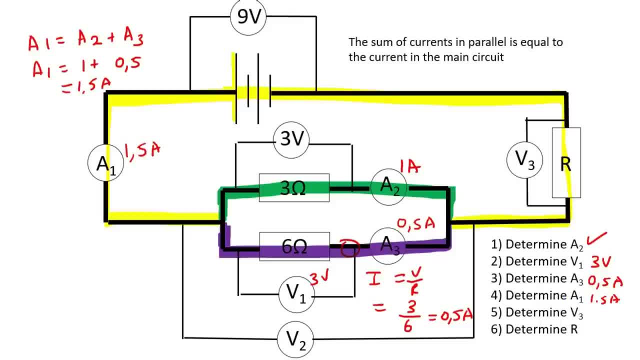 So A1 is going to be 1,5 amps. Now that's part of the main circuit. okay, which is the part in yellow. The next one says that determine V3.. Okay, Now we know the current going through here. 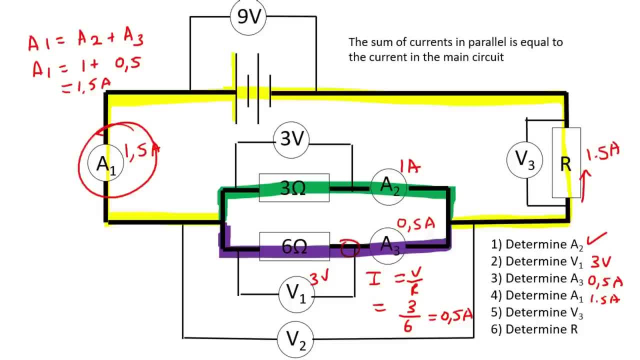 The current going through here would be 1.5 amps, because current in series is exactly the same. But the problem is we don't know this resistor, We don't have that resistor, So we're not going to be able to use. I equals to V over R or V equals to I times R. 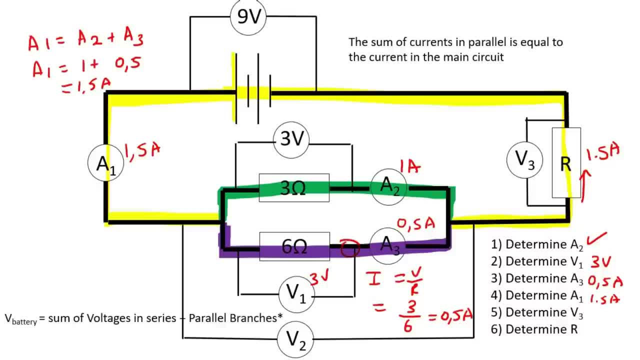 That won't work. But what we can do is we can look at this formula over here. So we know that the battery's voltage is the sum of all of the voltages in series plus all of the parallel branches, So the voltage of the battery is 9.. 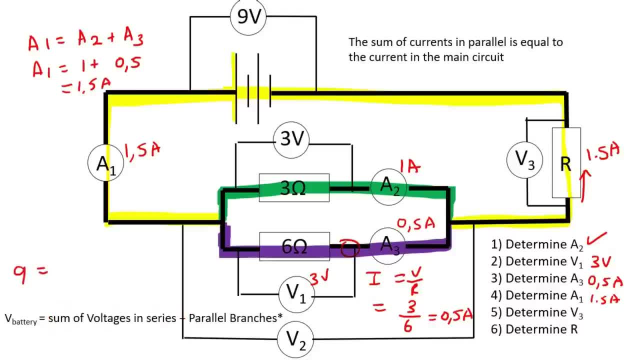 Okay, So we've got that. Now the voltage is in series. Now we actually do have a voltage in series. It's called V3.. And then the parallel branches. remember, you only take one of them, So they're all going to have a value of 3 volts.